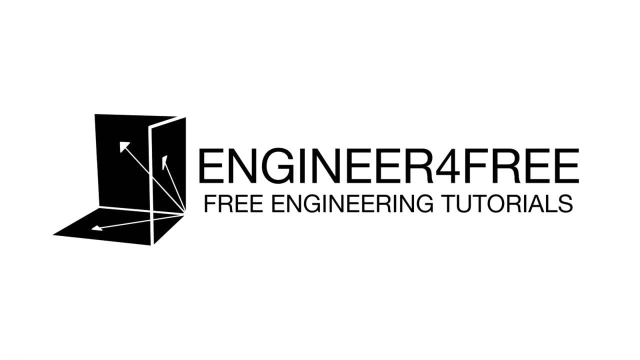 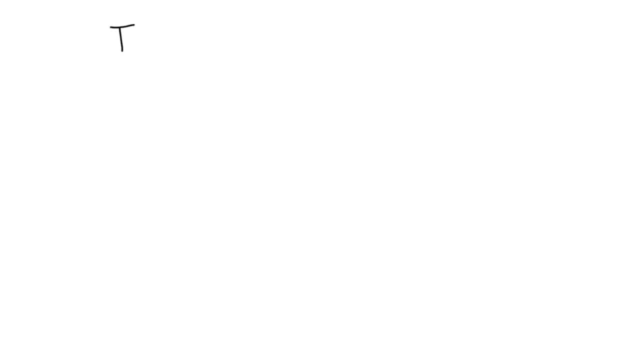 Hey, welcome back In this video. I just want to go over an example using the conservation of energy equation. It's also referred to as a conservation of mechanical energy equation, if you've heard it that way before. So it's just simply T1 plus V1, that is kinetic energy, and 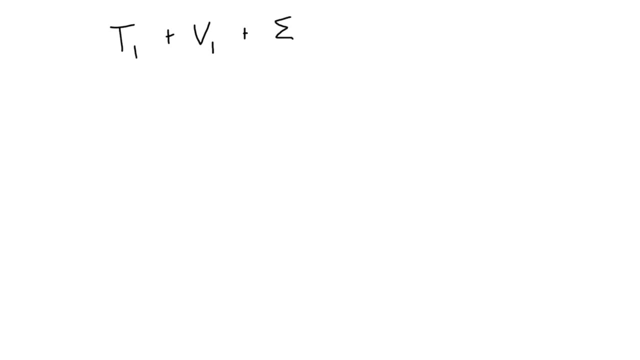 potential energy plus the sum of work done from state 1 to 2 is going to be equal to T2 plus V2.. So all this is saying is we just have our energy at state 1, plus or minus the work done on the object is going to equal the energy at state 2.. This work term right here is referring 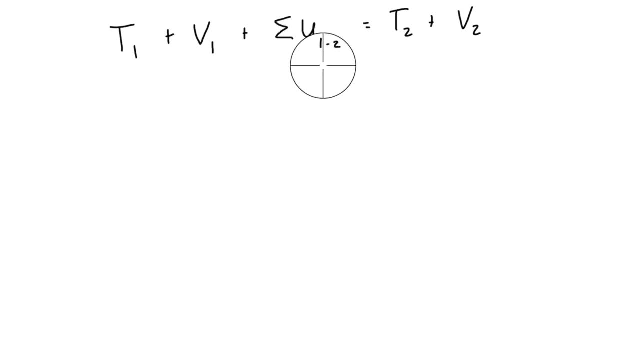 to non-conservative forces, which in our case, is basically always going to be friction. So if there's no friction present in the problem, that will drop off and this expression can simply just be written as: T1 plus V1 is equal to T2 plus V2.. So let's set up an example here. that's: 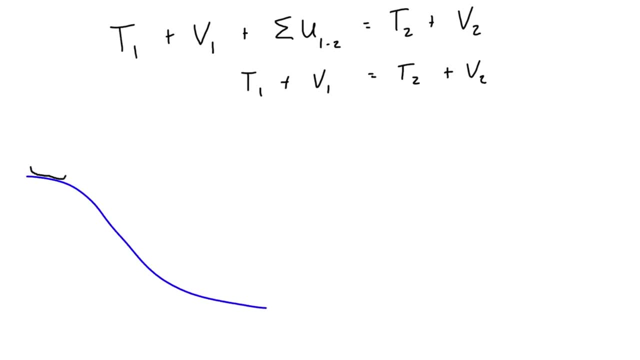 not going to involve friction. Let's say we have a guy snowballing. He's going down an icy slope, So let's give some values here. Let's say his initial velocity is going to be three meters per second. He's at a height here. He's going down a slope that's 10. 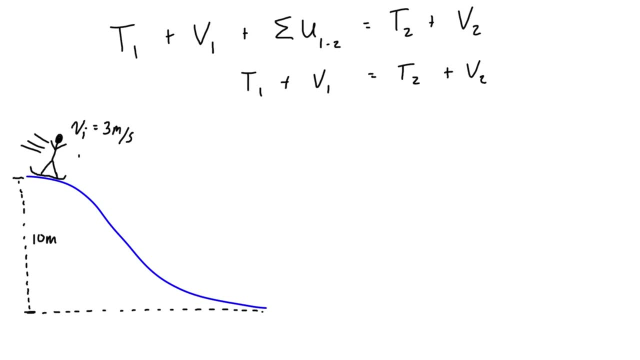 meters. We can give him a mass, but you'll see that it's going to drop out in a second. But yeah, let's say that this person is 75 kilograms and that the surface that he's going on has no friction. Now, that's clearly a simplification, but you're often going to see problems with 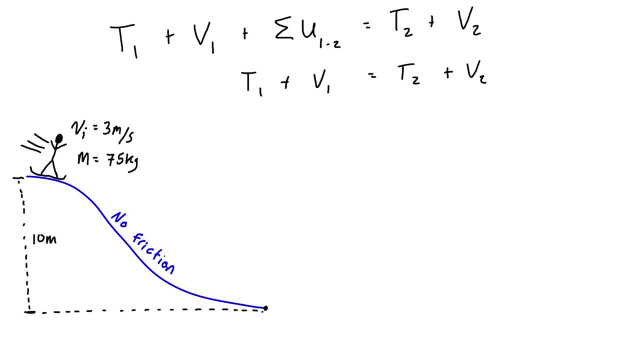 that simplification at this level, And then we're going to ask for his final velocity VF when he reaches the sum point, that is, 10 meters vertically below where he started. We're also not actually going to need the path length, because we're only dealing 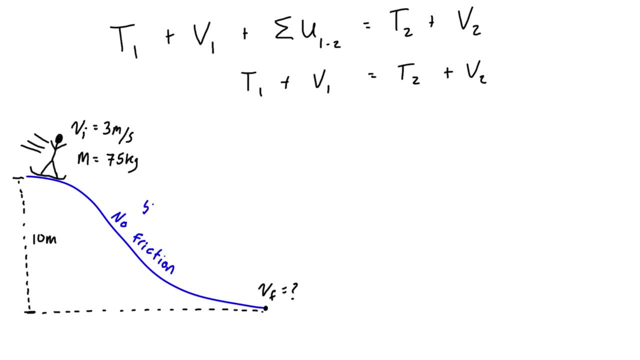 with the conservative forces of his weight. But if you wanted to, we can add in one that we won't need in this video. but we could just say that the path length that he travels- what I mean by that- is literally the length of the blue line. Let's call that 50 meters, because in the next 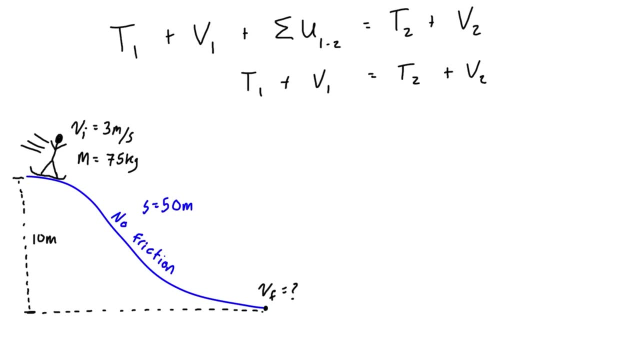 video. I'm going to go over this example with friction, So at least we'll have all these values here for the next video in the series. Okay, so we can just go in and fill out the expression kinetic energy at point one. it's just going to be one half m v, one squared, that's a lowercase v. 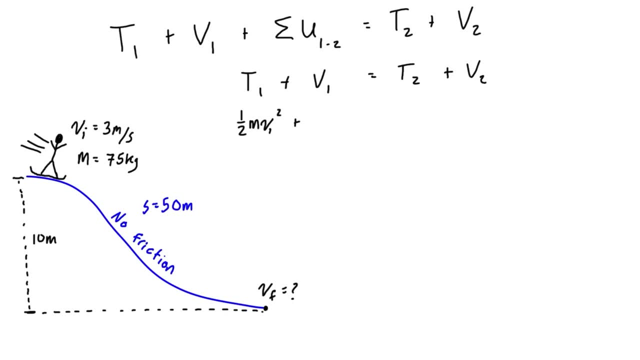 for velocity And then for gravitational potential energy. it's just m, g, h, mass times, gravity times the height, And the height difference in this case is going to be 10 meters, because we're going to have this point at the bottom, the height two. we're going to be setting that as a zero reference. 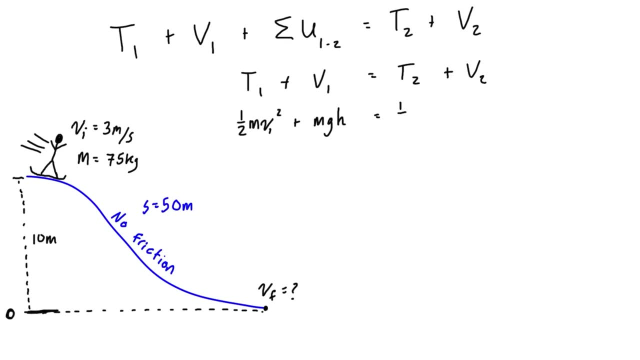 Anyways, carrying on, we can write our expression for kinetic energy: two, so that's going to be one half m v two squared plus m, g, h two, Alright, so right away we can see that all of the masses are going to drop out. we can divide both sides by m and they're going to be gone. And because h two is, 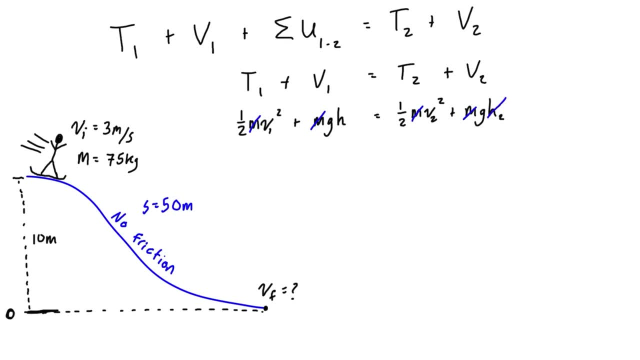 zero and h one is 10, this whole term. well, that variable is zero and basically the whole term is going to go to zero. So it's all going to drop off. So we can fill in the values that we do have left over. So we have. 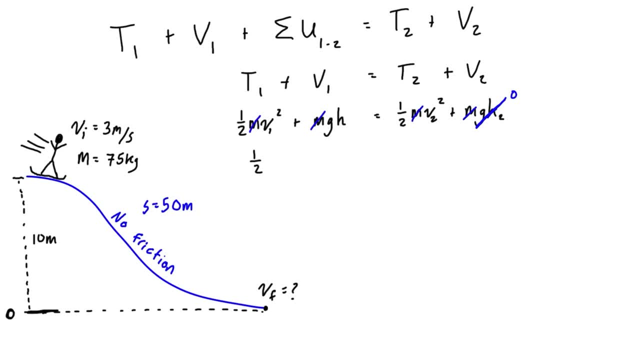 one half v, one squared, that is three meters per second all squared, plus acceleration due to gravity, which is 9.81 meters per second squared times height. So height in this case is what we're looking at here. it is 10 meters, it is 10 meters above. 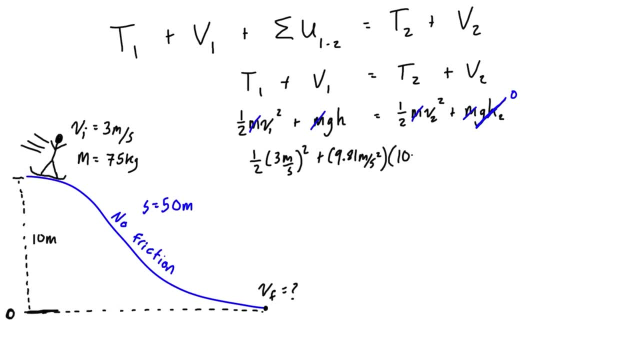 the reference zero that we're taking. So that's times 10 meters. And then on the right hand side we just had left over for what we had for kinetic energy: two. So we just have one half times v two squared v two is the unknown that we're looking for. Alright, so we can simplify these a little. 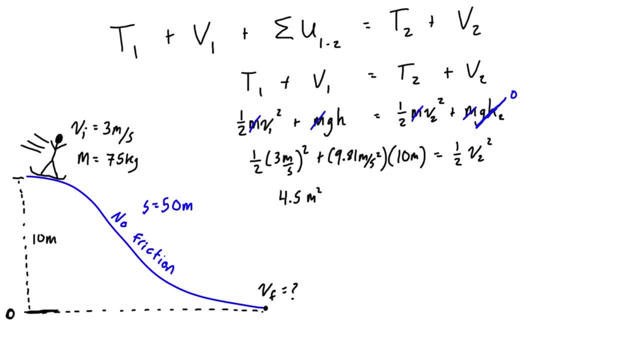 bit. we're going to get 4.5 meters squared per second squared, plus 98.1 meters squared per second squared is equal to one half v two squared. So the left hand side simplifies to 102.6 meters squared per second squared, which